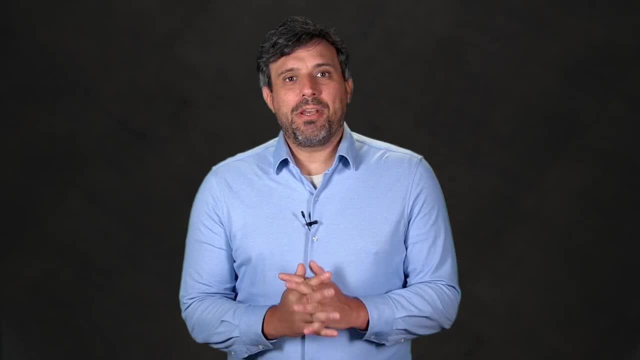 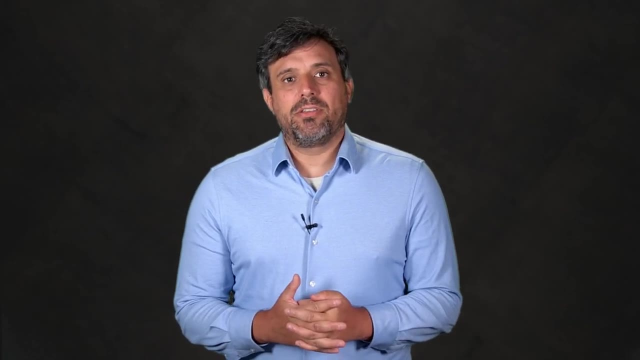 Land use might seem like a self-explanatory term, but it has a very specific definition with immense consequences for the way we live, work and go about our daily lives. Everywhere we look, the use of land is highly regulated and in the United States the use 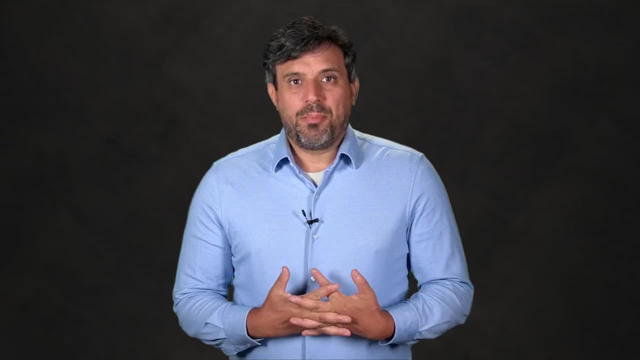 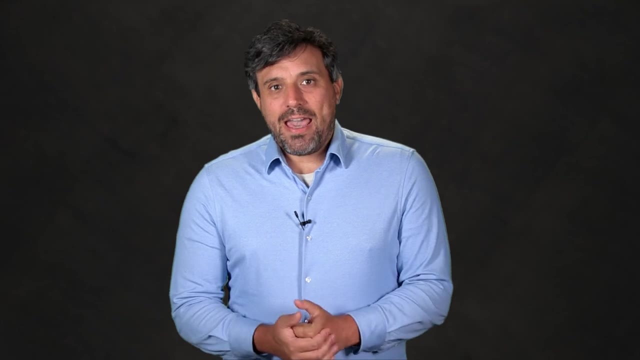 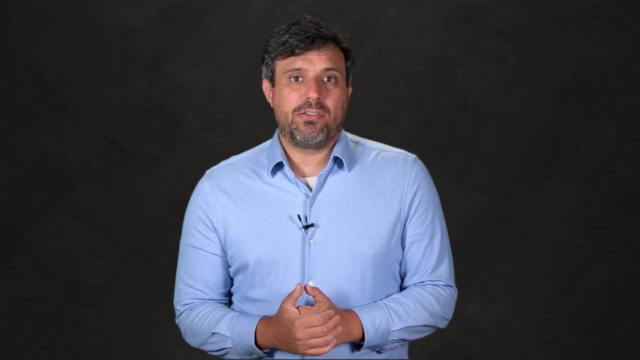 of land is regulated at every level of government, But the regulation of land uses is most conspicuous and most consequential at the local level. In fact, land use is the central concept for planning, as it's been practiced for over a century in the United States. Every kind of 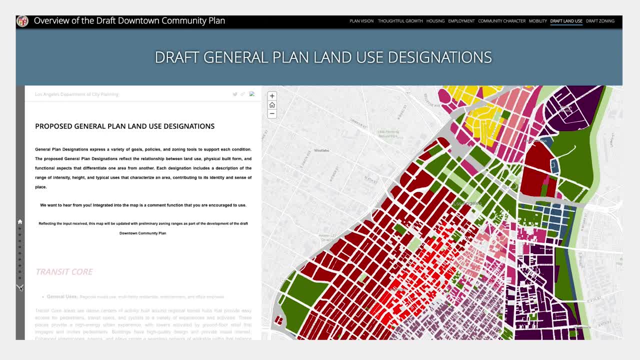 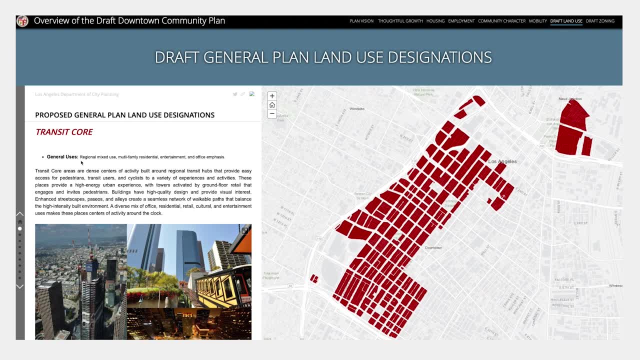 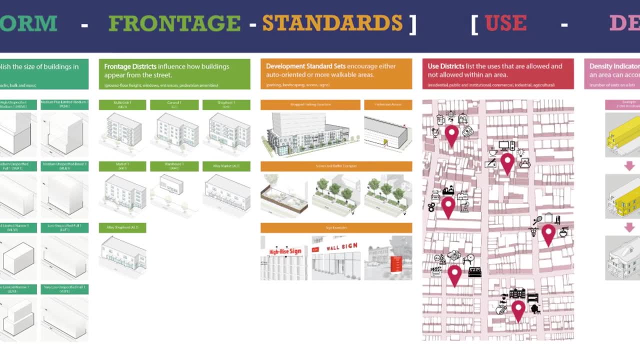 plan created by planning departments at the city and county level around the United States decides the future of land, whether that means comprehensive plans, general plans, community plans, etc, etc. Zoning codes are then used as the legal tool to enforce and implement those land uses. 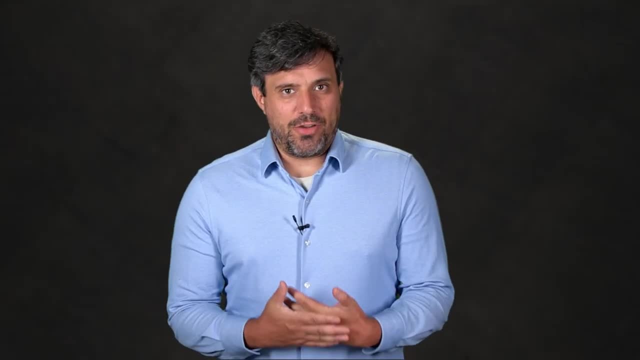 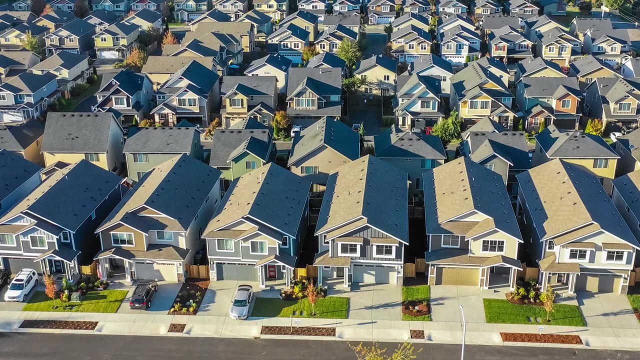 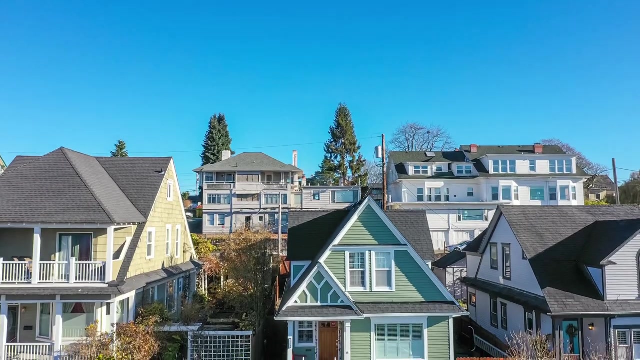 So far we've been talking about land use very abstractly, but to really understand the term we have to talk about some specific types of land uses. One of the most obvious kinds of land use is residential, which includes the houses, apartments and condominiums that. 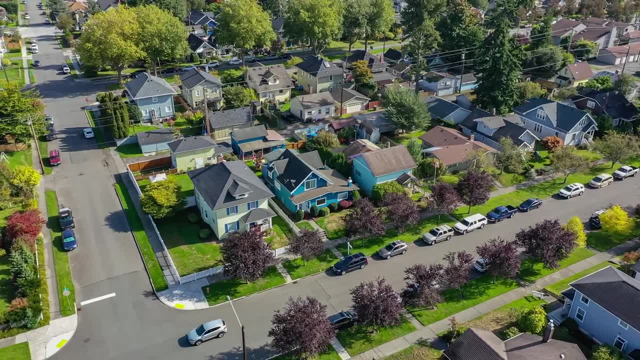 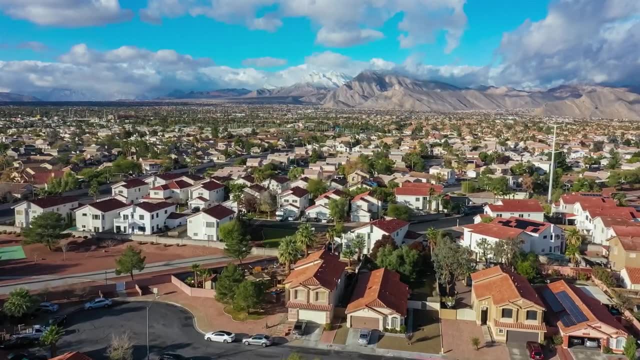 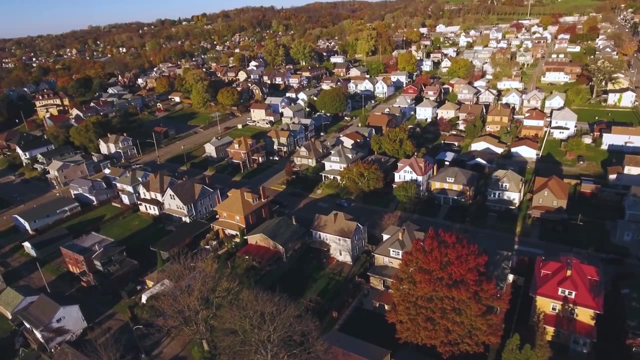 we think of when we think of home. Most cities in the United States are, by design, dominated by residential land uses. Moreover, most of the residential housing allowed in most of the United States is land use. The United States consists entirely of single-family detached homes, the homes with yards and two-car 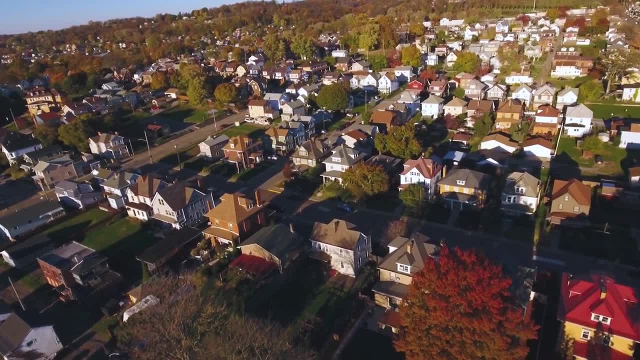 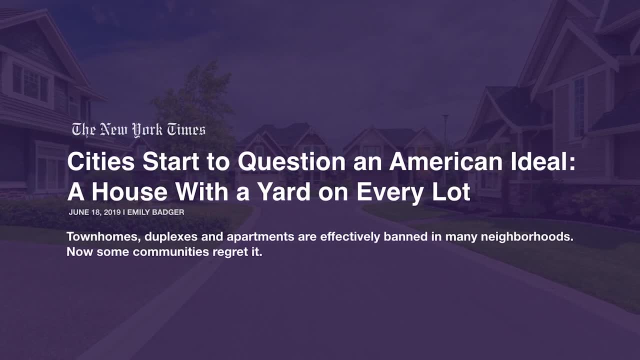 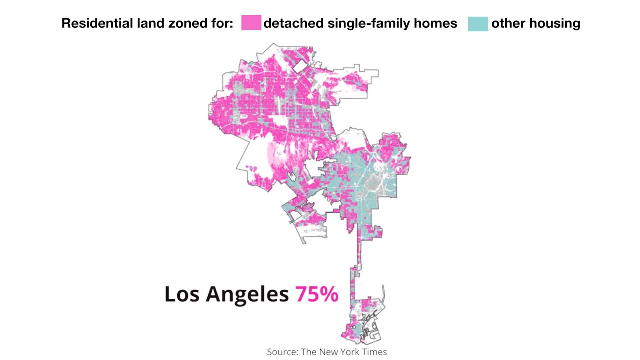 garages that are most commonly associated with suburbia. An article published by the New York Times in June 2019 quantified the amount of land devoted entirely to residential uses. In Los Angeles, for example, 75% of the city is zoned exclusively for single-family. 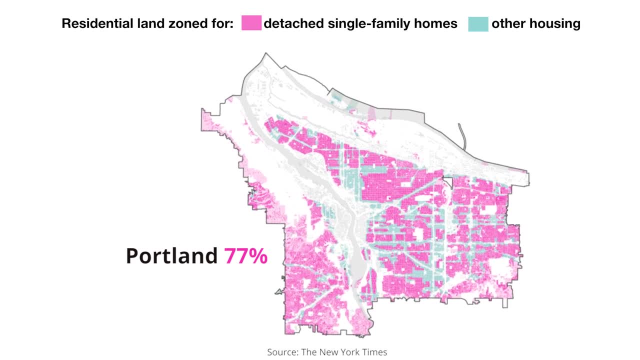 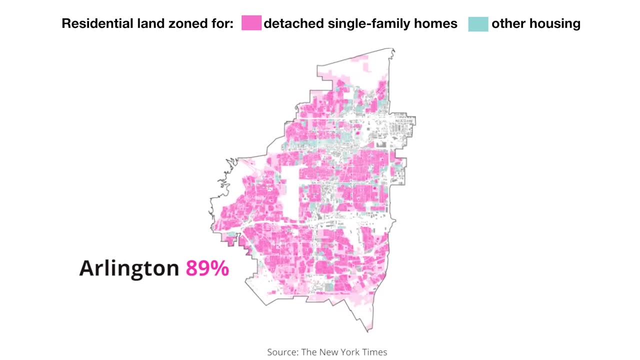 residential uses In Portland, Oregon. it's 75% In the United States. it's 75% In the United States. it's 77% In Charlotte, North Carolina. it's 84% In Arlington, Texas. it's. 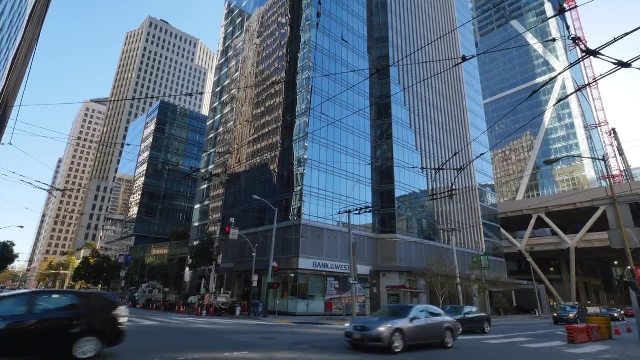 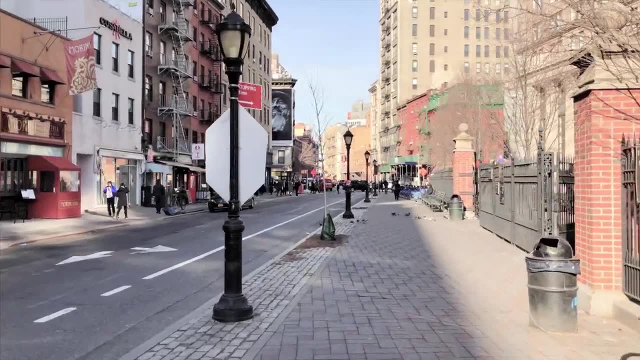 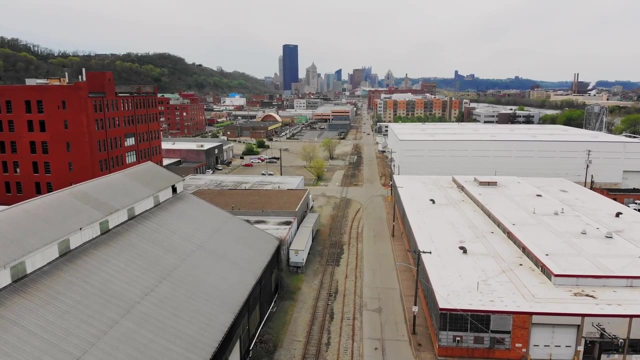 89%. Other common and easily recognizable land use types include commercial and industrial. When some combination of uses is allowed in neighborhoods or on individual parcels, it's called mixed use. Land use planning has its origins in the desire to separate residential neighborhoods from the pollution created by industrial businesses.